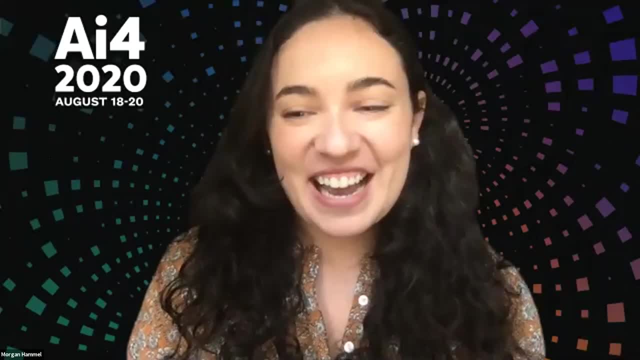 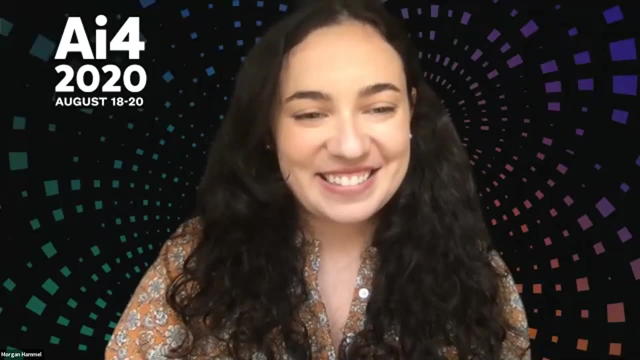 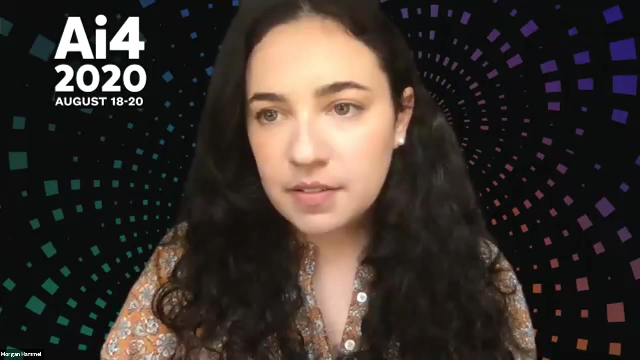 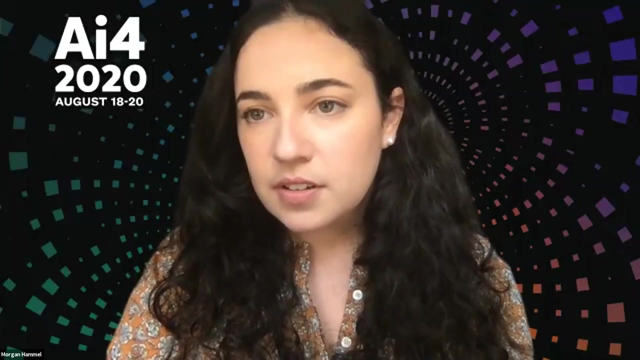 to our virtual stage. Meltem, you can come on up, Okay, great. So I'm going to turn my camera off and you can start sharing your slides and take it away. Hold on, We can't hear you, Meltem, Is your mic on? My mic is on. There we go. Okay, we can hear you. 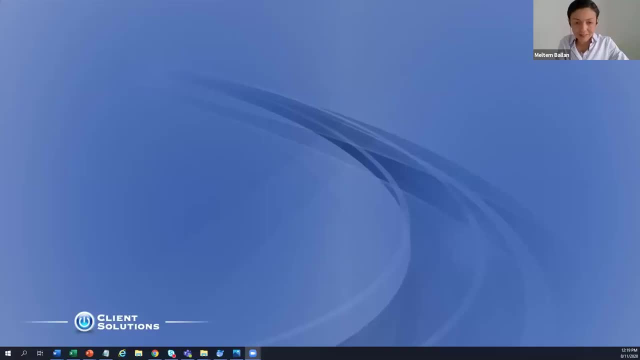 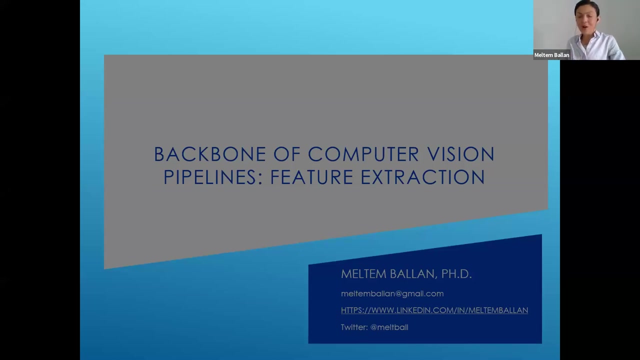 Awesome Screen sharing had a little bit of a glitch. Sorry about that, But since we are going to talk about technology today, we can forgive that. So, hi everybody. This is Meltem Balan. I work for General Motors as a Data Science Fellow, But before I joined, 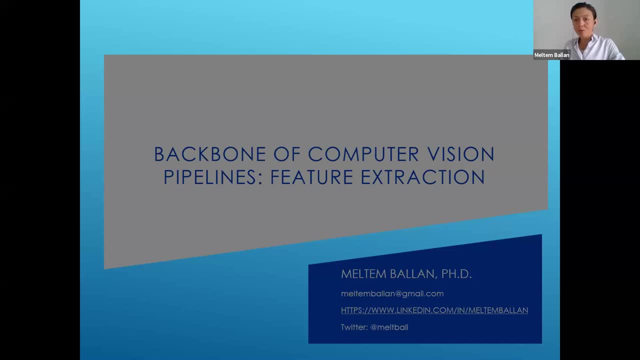 GM. I spent two decades working on computers. I have been working on computer vision and image processing problems, both as an engineer and a computational neuroscientist. First of all, I would like to thank organizers for the invitation and welcome you to my home office. The most important part of computer. 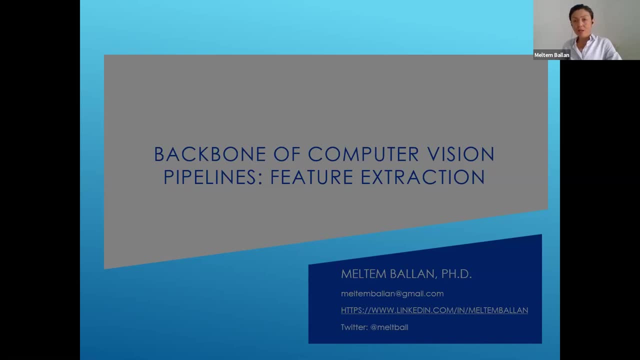 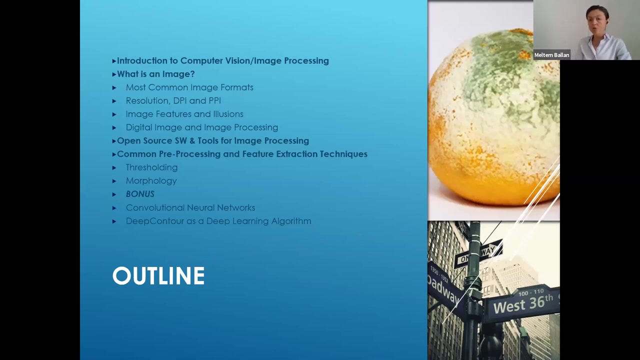 vision is feature extraction. The vast majority of algorithms are developed around extracting best representative features of objects. Today I will deep dive into those features and the feature extraction techniques. Let's start with outlining today's talk. I'll give an intro to image processing. I'll give 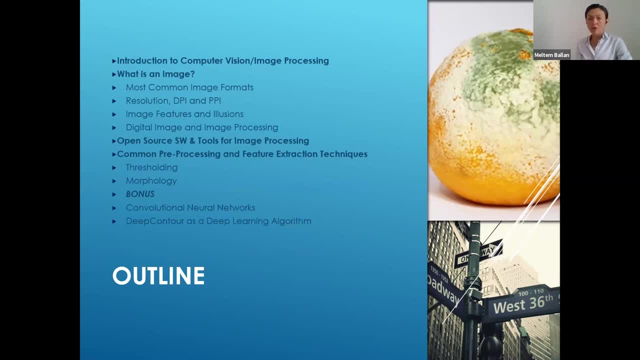 you a little bit about history, the story behind the most referred image in the discipline, most common image formats and definition on an image in details. My goal is to show you the important points of the image processing process And I'm going to talk a little bit. about the details of the image processing process. In this video, I'll show you how you can get the most accurate image on an image. This is what I talked about when I said the most accurate image on an image. in the example of text. I'd like to start with an actual. 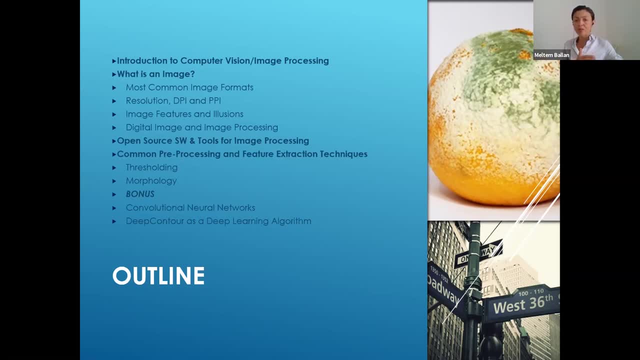 the human perspective and also computer's perspective of the image. So I will touch base to some techniques used in physics, visual cortex studies and psychology. Later I will provide some common tools, depending on your background and where you are at in your career. 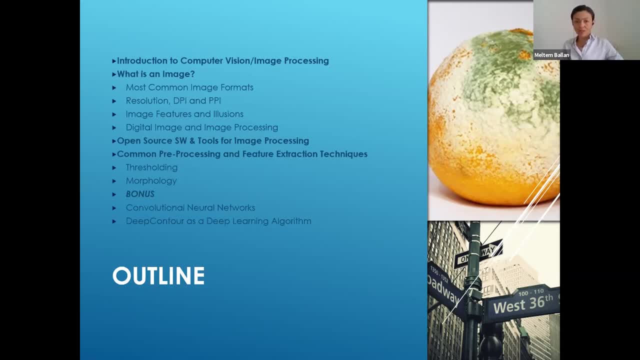 I will then touch base to thresholding and morphology. The hope is to leave you with a laundry list of items involved in computer vision, so that I'm leaving you with a bonus part of my talk: that you can see the full cycle of a computer vision project and you can implement it by yourself. 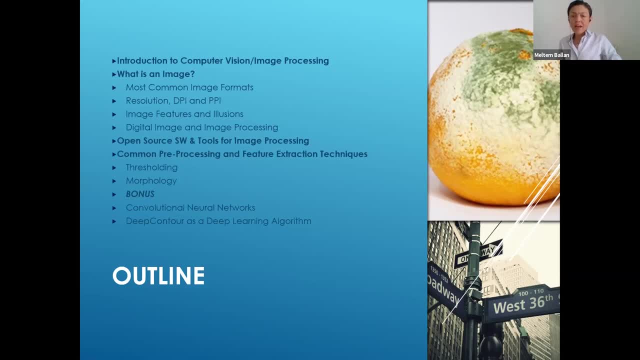 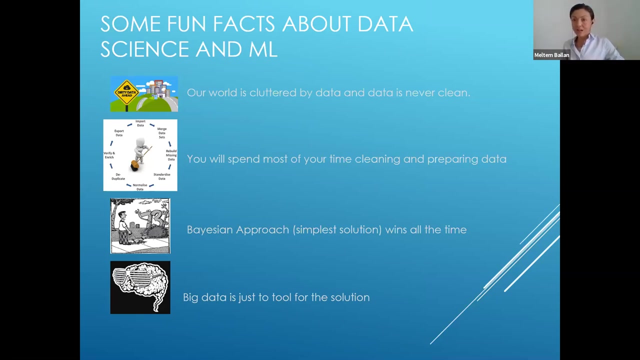 All in all, I wanted to show you what has been done in the field and the future of possible, the art of possible. Oh, this is not a trick slide, but rather important one. Today's topic is is the objects, and objects are also the data. There are four universal rules in data. Data is never clean. 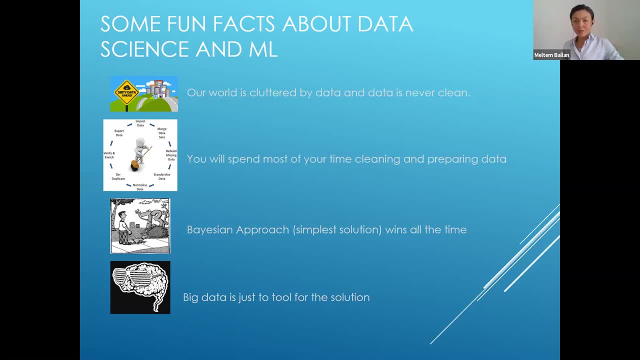 You will need to clean your data first. The simplest solutions are always the best solutions. Big data is just a tool, not an answer to data. So let's see how far we can go today with our particular data images and feature extraction. Let's begin with the introduction. 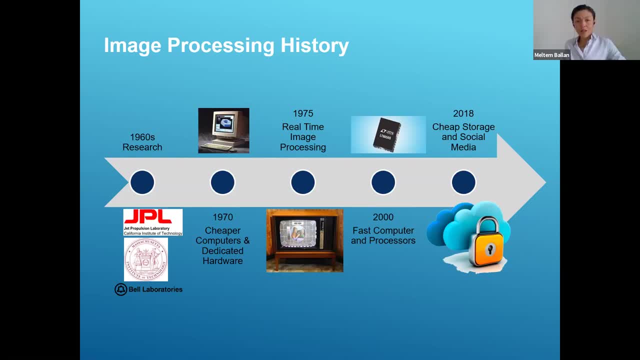 I believe that POS is the reflection of the future and it is no different in the computer vision. Technology is constantly affecting the change in the computer vision while, while evolving within, Second World War was one of the biggest triggers moving technology forward, For example, JPL, MIT and Bell Laboratories. 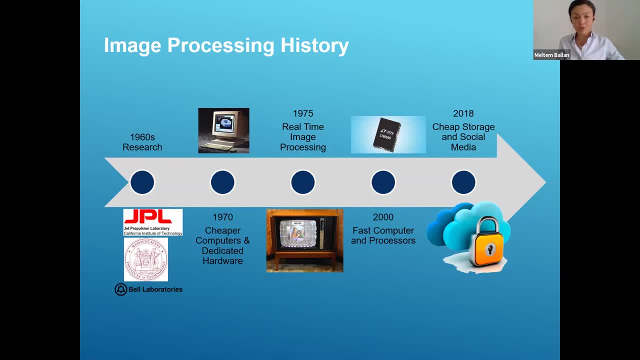 were developing communication and internet technologies for military and eventually became available for us to use in 1970s. Real-time information processing became possible in 1975 and we were able to watch color TV. 2000s were the years that we met the fast computers. 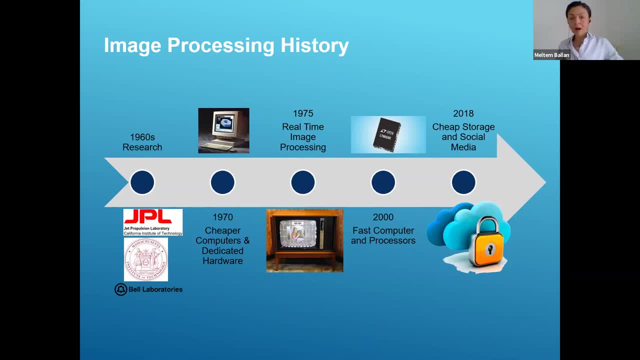 and computers became part of our lives. We started to play computer games Last several years. cloud became available for everybody and IoT became part of our daily lives. We all use Instagrams, we all use Facebook and everything all together we have a lot of images. 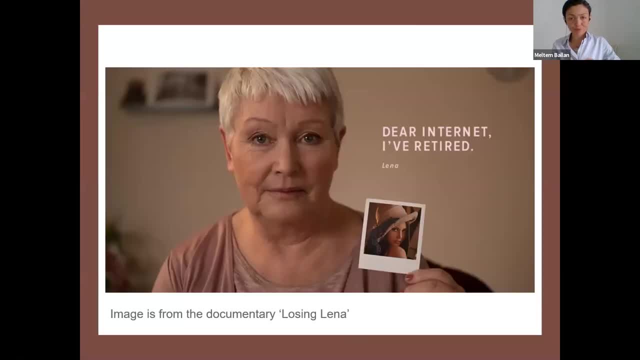 digital images shared on those platforms. But before, since we are talking about computer vision, we have to definitely talk about Lena. Lena is a symbol of an era. There are goods and bads between the lines of this image. The picture was taken by a Playboy photographer. 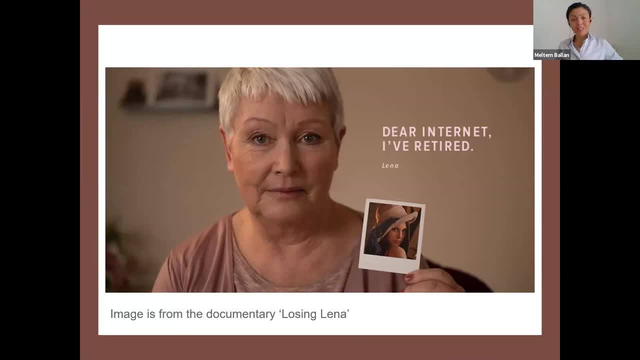 and published in the magazine in 1960. Later it became the most iconic picture in the computer vision. Computer scientists, neuroscientists, psychologists, psychiatrists has been using this image since 1973. The significance is that it was a human face and glossy with a little bit of black and white. It was a human face and glossy with a little bit of black and white. It was a human face and glossy with a little bit of black and white. So the image has a lot of contrast and lines. 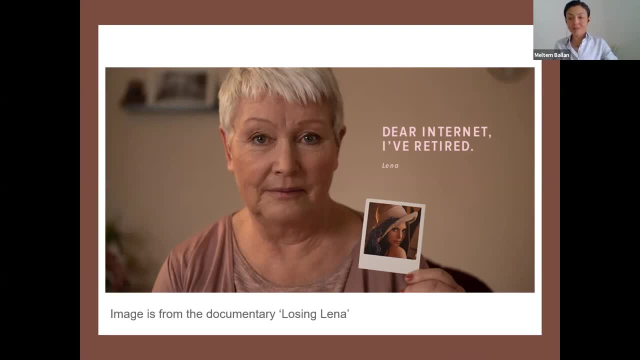 Since then it has been used as the standard test image for computer vision, biologically motivated image processing, like retina studies and robot vision. She revealed the story of this particular image that she's holding here in 1997 at the 15th Annual Conference of the Society of Image Sciences. 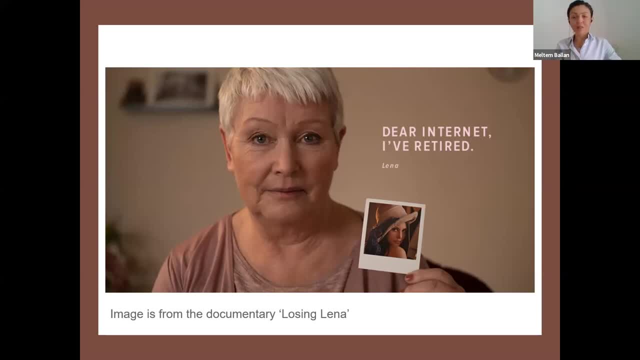 science and technology. Admittedly, I didn't know the story until then. When we talk about attractive women in computer vision and image processing, it is also worth to remember Kodak Shorleys. Not too surprising, one of the Shorleys was again Lena. 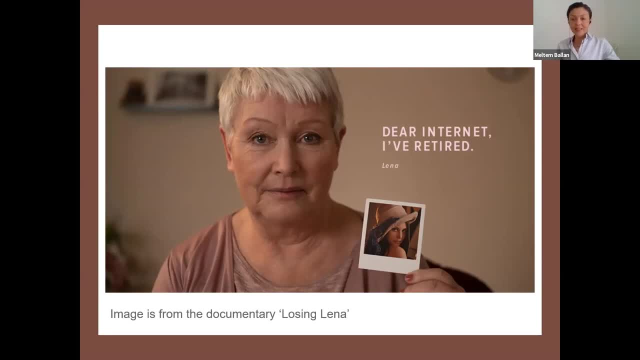 Throughout my career, I had mixed feelings. Most definitely, she's the most used when it comes to image processing and colors, And I use this image over and over throughout my two decades career. It has been only the last 10 years. the gender bias has been discussed around this picture. 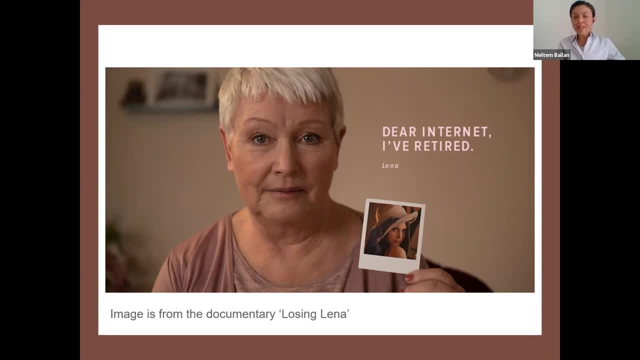 Once again, Lena is front and center. I definitely learned from her picture over the course of my career. The contour and flat edges represent how we process and identify objects and then name it. I definitely felt lonely in the engineering classes and had questions about this picture. 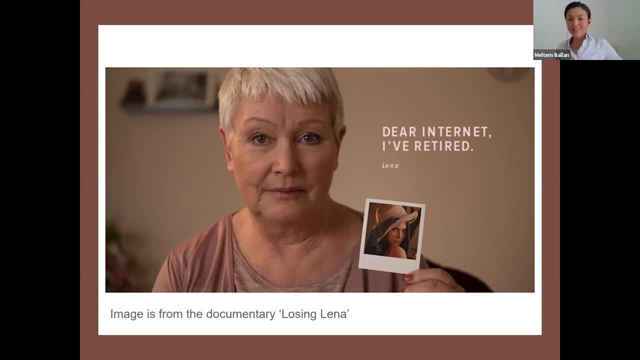 I'm also an advocate for growing women in data science and STEM. But again, Lena wrote a history and led computer science to the point we are at. I will use Lena in this talk in the following slides. It is again up to you to decide. 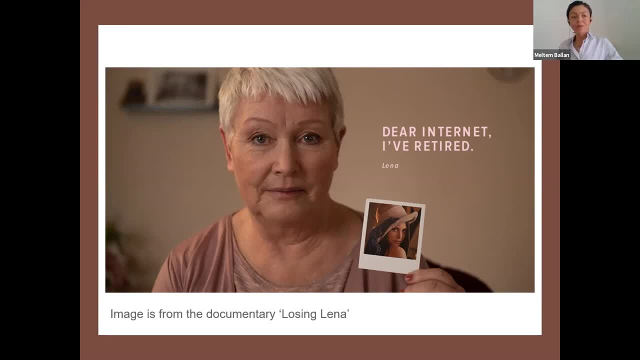 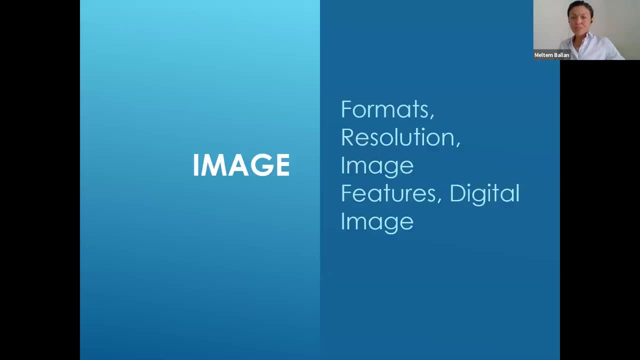 how you will test and implement your algorithms, And I definitely suggest you to go see the documentary about this. I want to start with the basics of image. The definition of image we will discuss today is a picture that has been taken, scanned or copied and stored in databases or in the cloud. 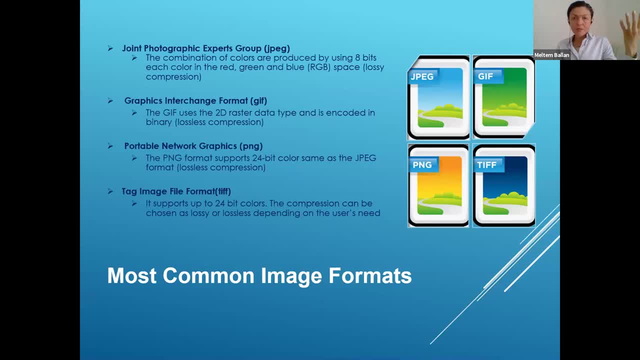 There are four main formats That I want to include here. First of all, JPEGs. They are stored in 16 million- 16 million colors. The combination of colors are produced by using eight bits each color in red, red, green and blue. 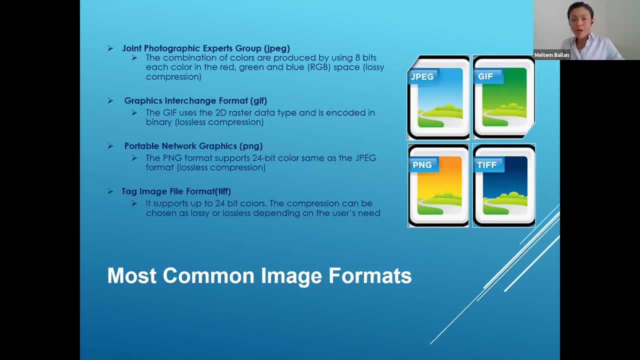 The compression is 10 times more powerful than bitmap to store images without degradation. However, high compression rate might cause noticeable noise and quality issues in the image. GIF format is better to store images with text. GIF uses lossless compression that does not degrade the quality of an image. 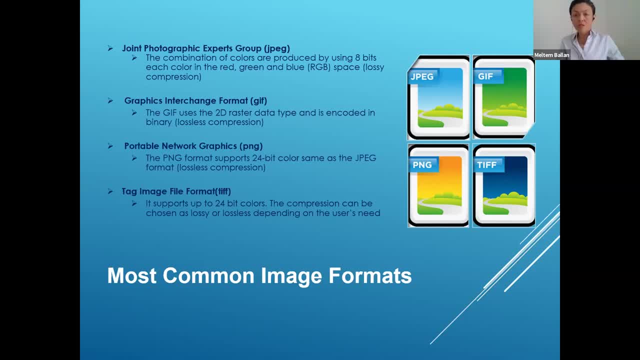 However, GIFs can only store images of 256 colors. GIF supports animations by storing a stream of images in a single line. PNG can be described as the more developed version of the GIF. The PNG format supports 24 bit colors, same as JPEG format. 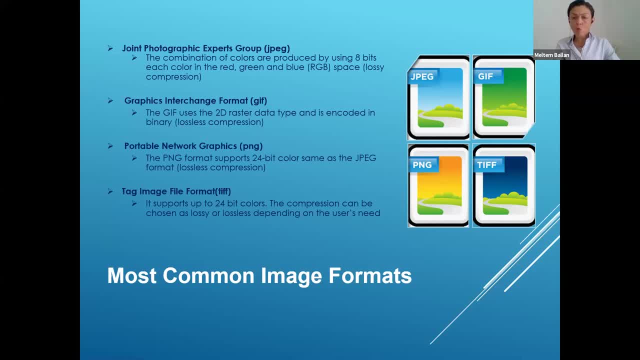 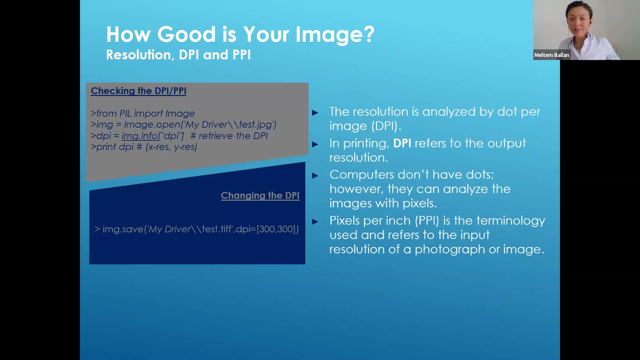 Therefore, PNG image may include over 16 million colors. TIFF supports up to 24 bit colors. The compression can be chosen as lossy and lossless, depending on the user's needs. So this is important to know the format of the image to gauge what the limits and needs are. 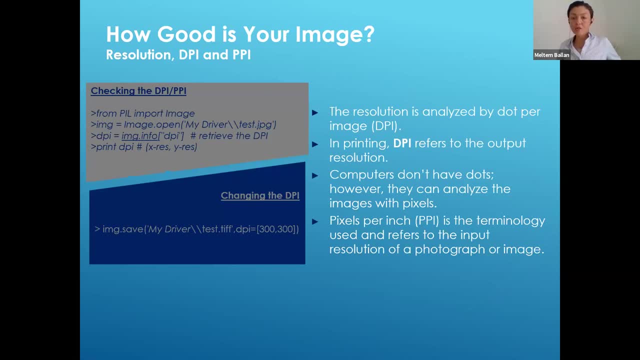 However, the resolution of an image is essential to start your analysis. The resolution is defined by dot per image In printing, DPI refers to the output resolution. Computers don't have dots. However, they can analyze the images with pixels. Pixels per inch. 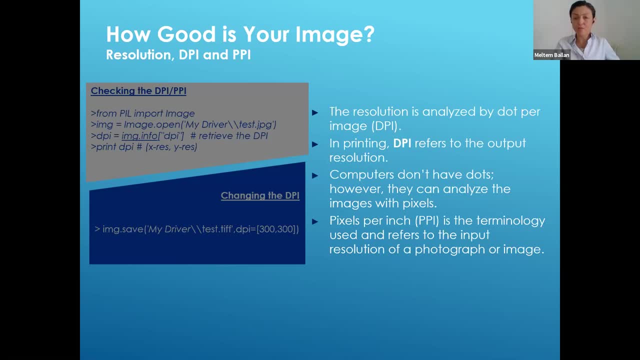 is the terminal that you use and refers to the input resolution of a photograph or image in computer vision. So nowadays we use DPI and PPI interchangeably. You can always check and see the DPI and PPI of your image and also adjust it to your needs as the first step of feature extraction. 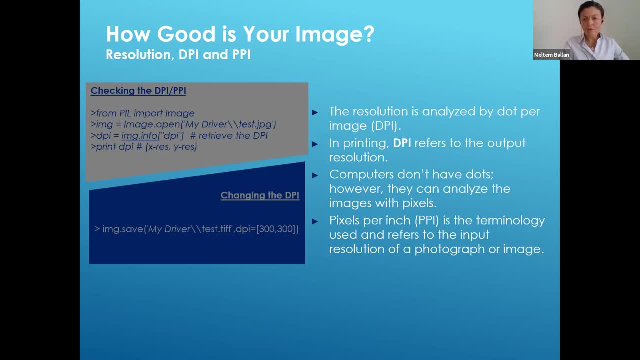 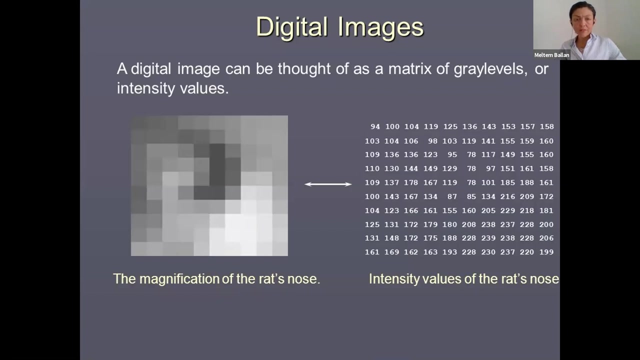 I will be silent For a sec for you to check and see how you can actually check the DPI and PPI and change the DPI. And again, I used Python here. The basic library PIL is used here. So let's begin with the digital image. Images can be a picture with a background. 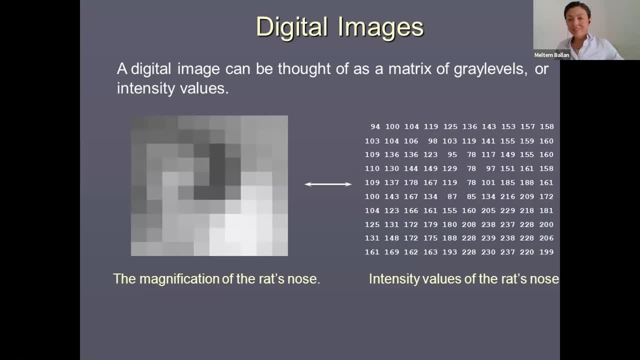 text, a picture taken from an accident, money, transcripts, animal pictures, nature pictures, scanner and printer outputs everything and anything that you can see with your eyes and process it, But when those are entered in the computers they become just numbers between zero and 200, 255, as shown here. 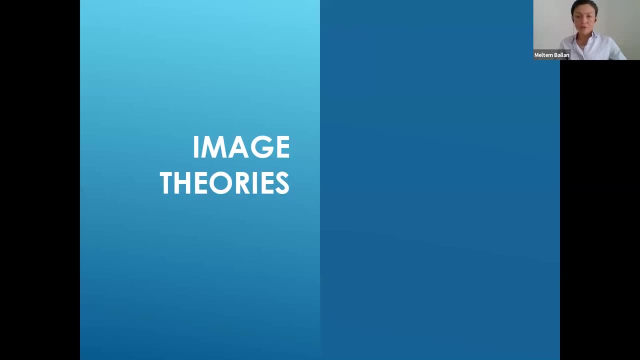 You heard me using image, computer vision and patterns up until now. Before I deep dive further, I want to clarify where I stand When it comes to image processing, computer vision and pattern recognition. these terms are all together. In your career, you will see a lot of these words coming together. 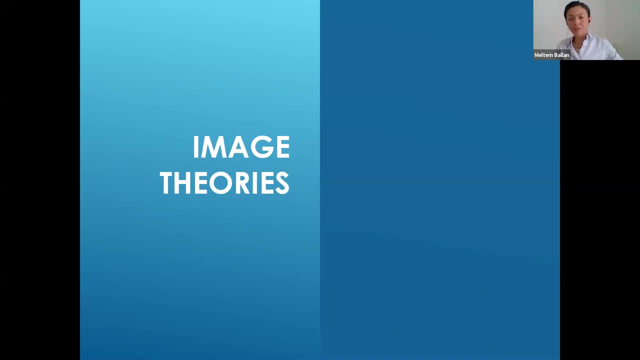 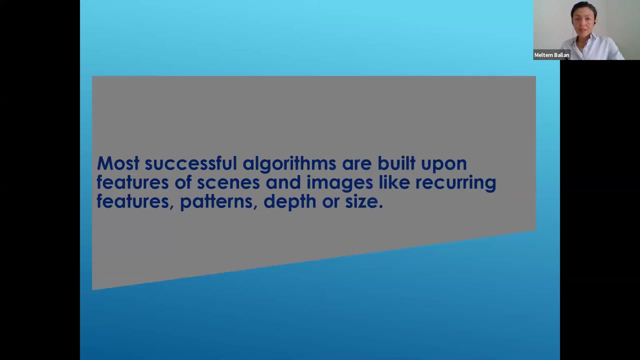 And it has been used interchangeably Between the disciplines. the closest disciplines, the computer regions I can see, are image processing and pattern recognition. I strongly believe that these terms are lined up together and the differentiators are very slim. if not, You will hear and see slides like this throughout my talk, as I want to provide. 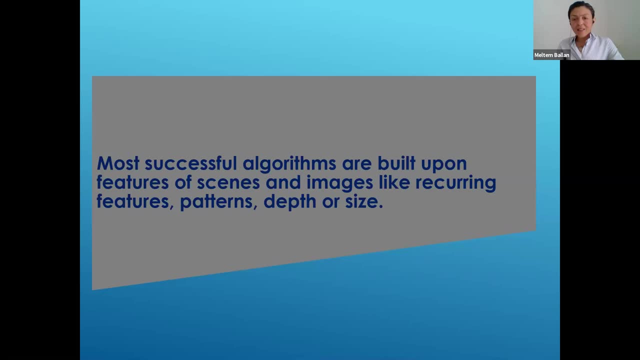 a whole picture within 25 minutes. The ultimate goal is to represent the objects as humans can see. So we computer scientists or manabees implement physics and psychology behind image processing. If nothing else, we use it to start conversation at a cocktail party. 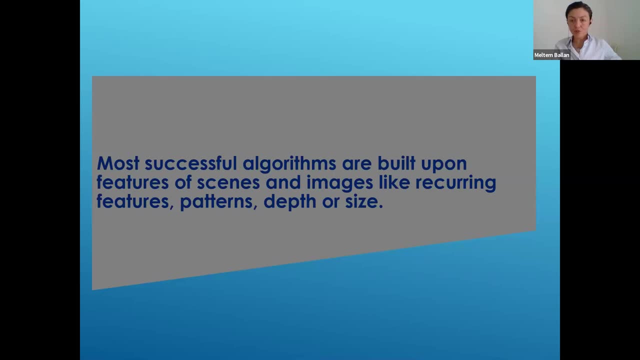 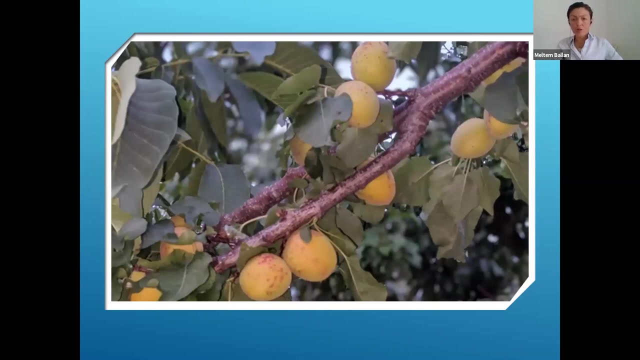 So let me tell you a little bit about fractals and illusions. I hope that you can actually start implementing these techniques. The images with repeating patterns and features are called fractal images. Two basic questions. we ask to identify if an image is fractal or non-fractal. 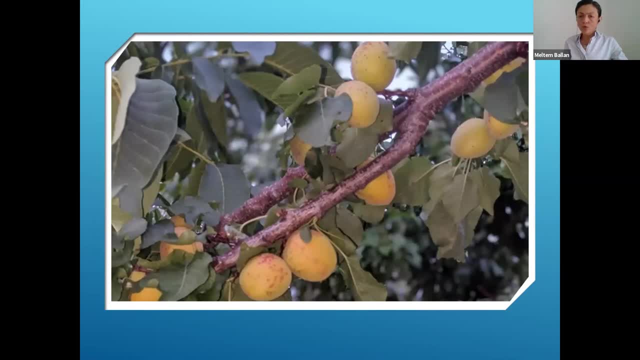 One. is there a new feature revealed when we put the image under a magnifying glass? Are there different sizes and scales of the same image? The leaves, the freckles on apricots and even the warm bites on the leaves are the fractals. 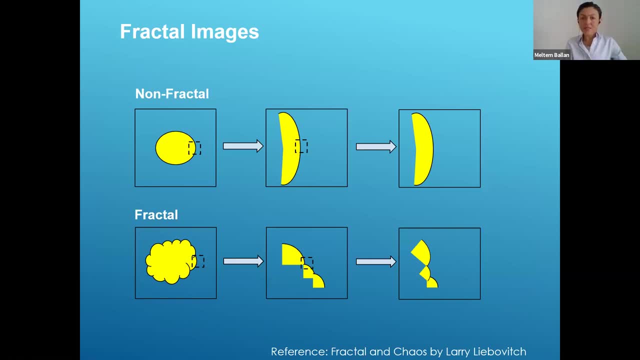 I'll try to explain the theory, as Larry taught during my PhD, but it is a complex topic and it will take take me more than 25 minutes to explain in details. I definitely suggest his book if you want to learn more about the fractals. 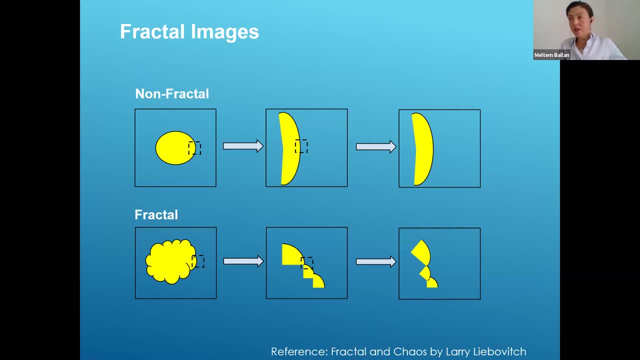 The technique is used to compress images or, in our case, for the feature extraction. Even though some of the features are lost during compression, fractal code can be used to recreate an image or extract the features. There are three main properties to remember. 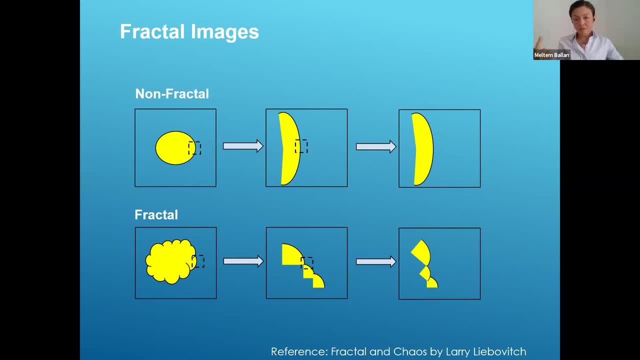 One is the self-similarity and the second one is scaling. And the last one is dimension, As it is shown in the picture. the image or the feature in the image can be enlarged by a window until the vehicle is resolved. Scaling provides the ratio of biggest and smallest spatial resolution. 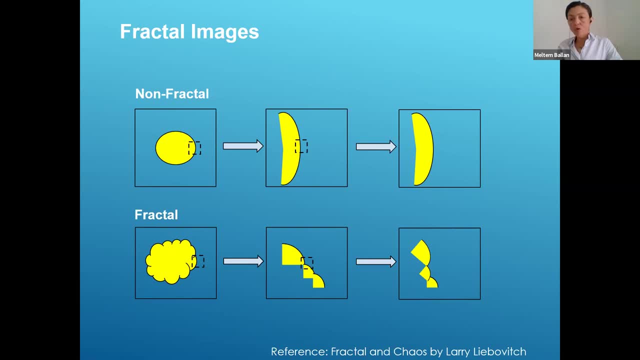 In other words, scaling basically reveals the number of divisions. Dimension provides the number of new features at the highest magnitudes, In other words, number of smallest shapes are called dimension. Hope this will give you some starting points so you can employ fractal coding for your AI algorithms in the future. 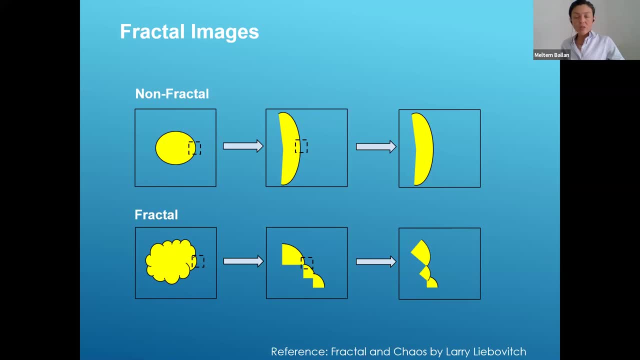 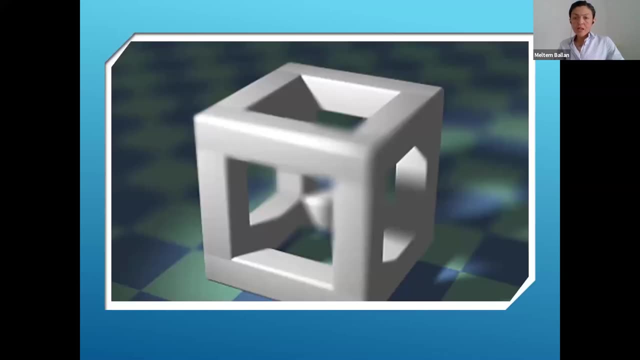 Oh, before I forgot, try quadtree decomposition or Huffman decomposition for an image that I showed here. Illusion is one of the terms which is borrowed from different health sciences: psychology, vision, ophthalmology. Hope that illusion will lead to the basic. 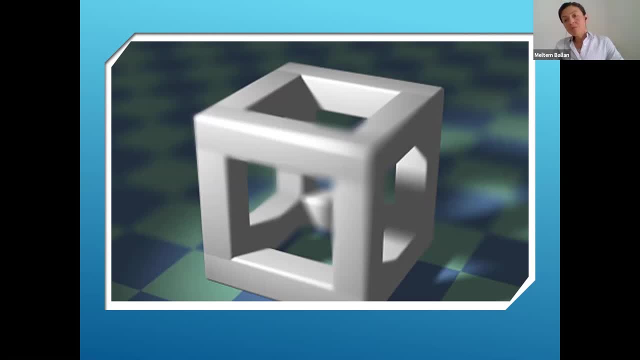 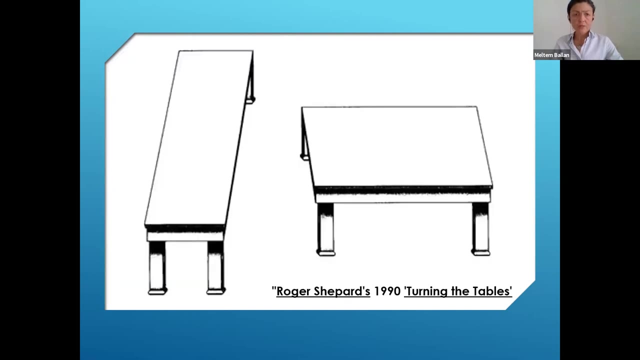 features on an image and geometry of the pieces of an image. Here I will limit my topics with the Shepard's table illusion, checker illusion and Amos room illusion. Let me start with the Shepard table illusion. One of the most used concepts is this particular picture here. 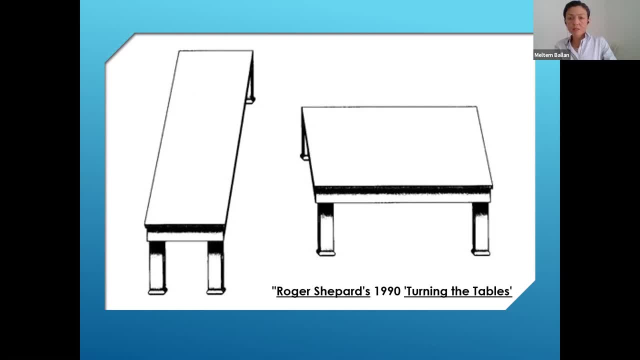 In Shepard's study, the table seems longer and thinner than the other one, even though it is actually identical to the other. The receding edges of the tables are seen as if stretched in depth. The table which looks like square is further away and appear wider. 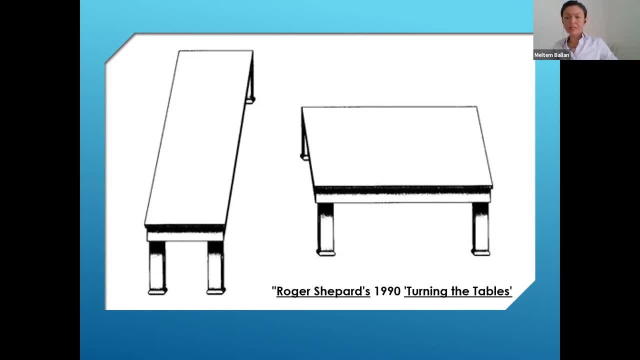 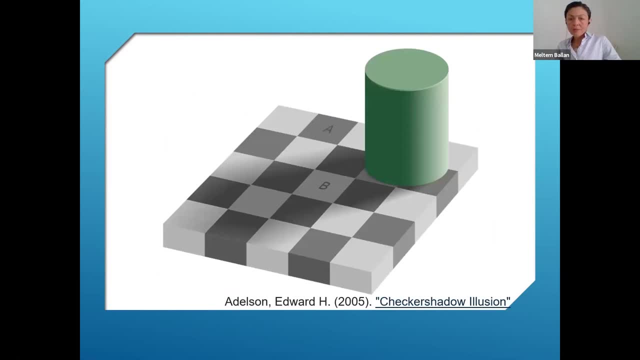 This tells us the power of depth in an image and how to represent in the computer. This is an example of the checker shadow illusion and it was first represented in 2005.. The green object is obviously shadowing the checkerboard object. Optical illusion of the shadows makes the upper left corner of the image darker. 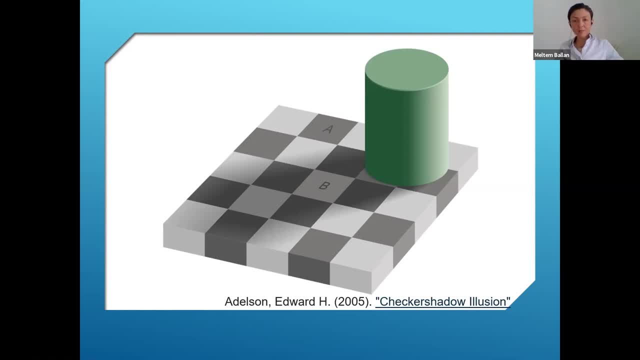 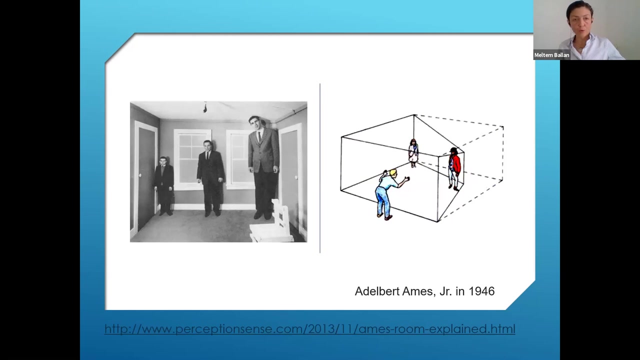 However, in reality, checkerboard has identical brightness for both gray and white squares. If you were to print the entire board, it will look identical. The last one, and most exciting one, is called Amos room. Don't you think that the man on the right is giant? 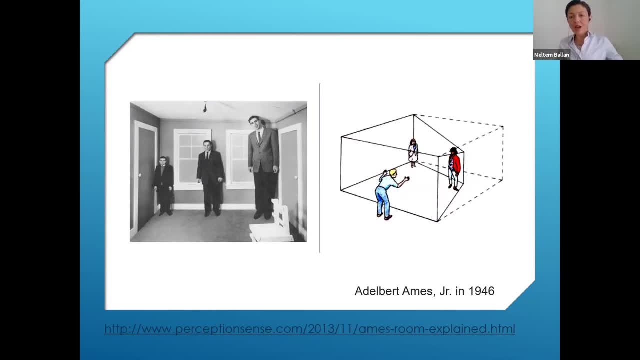 Is in fact the angle that you're looking at, and the giant man is much closer than others. to trick your eyes. The room is room. The man is actually almost a triangle. The person on the right corner is the closest to your eyes, Isn't it amazing? 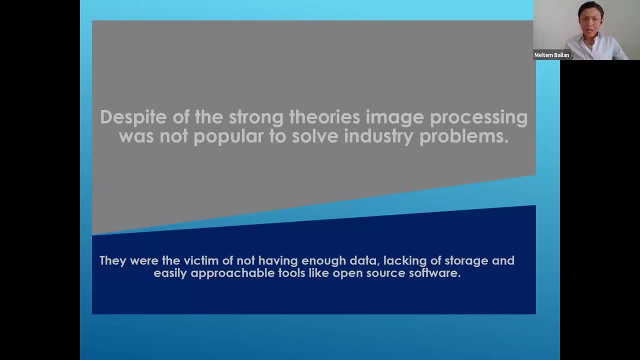 So these algorithms and the mathematical models have been developed since 1800,. however, they are the victims of not having enough data, Lacking the storage and lacking, lacking the computation power. So, oh, I was almost forget, forgetting power of the open source tools in this light. 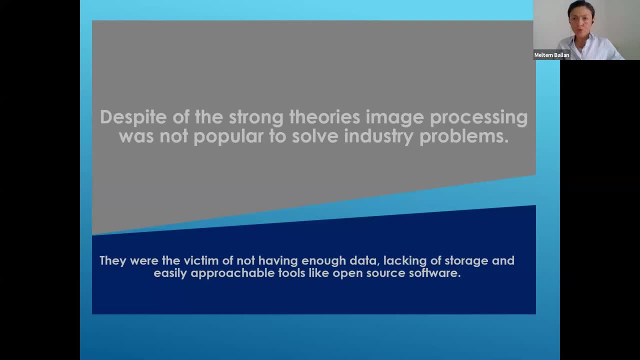 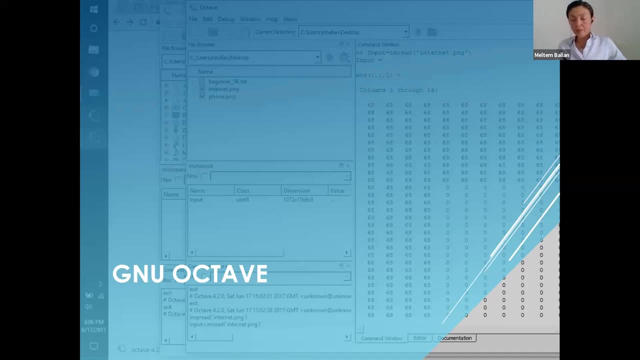 So let me start with some of the open source tools that you can actually implement. So one of the tools. if you're coming from academia, like me, and familiar with MATLAB, there is one of the tools that you want to start with it. It is: 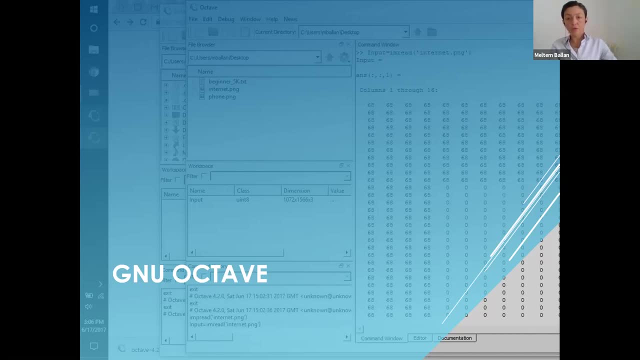 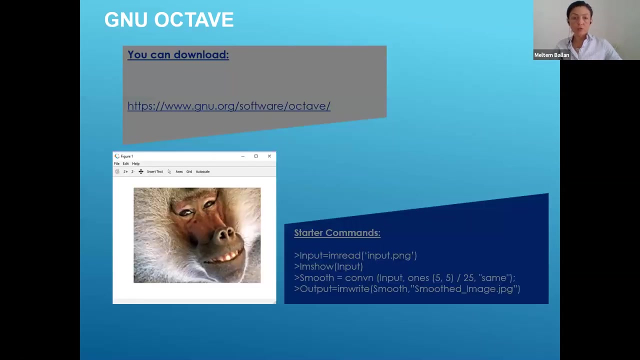 it is very powerful because it was developed for the numerical, numerical computation and number images that we're talking. as I showed, it's between one and two hundred fifty five. so this, this tool, is one of the best tools that you can start with. 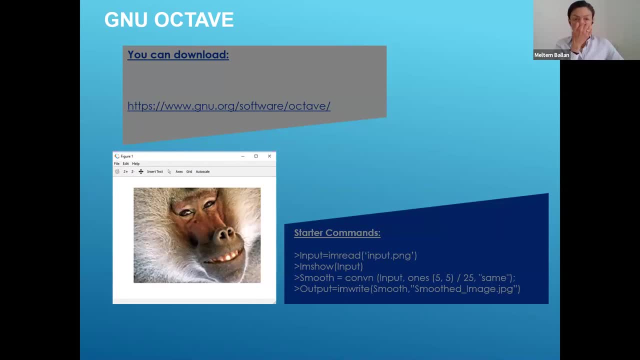 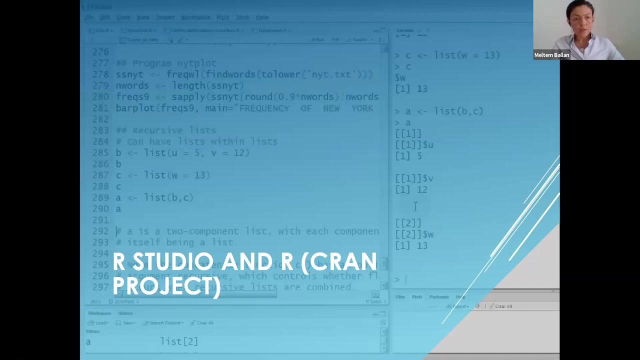 This is it. This is the starter slide that you can go down, note down note octave and start using some smoothing algorithms and then end up seeing this little friendly face here. So the other tool that you can actually use is R studio. R is a statistical tool that has been widely used. 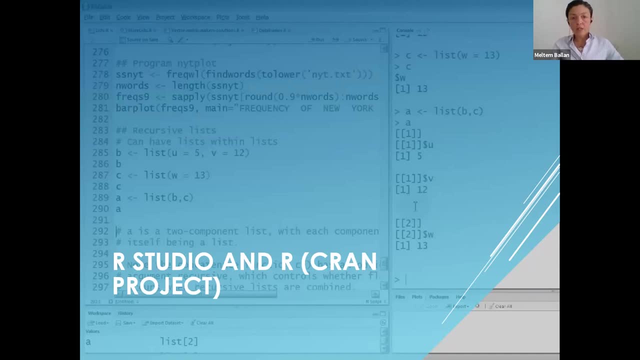 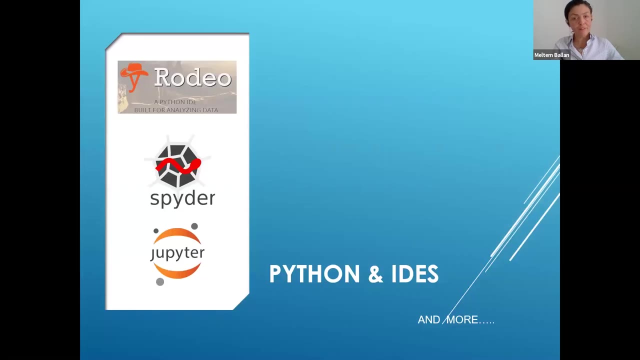 And I'm sure you heard about that, And they also have a lot. R also has a lot of image processing libraries for you to choose. My favorite is Python. Unlike R and Octave, Python is widely used general programming language. There are a lot of different ideas and libraries to use in Python. 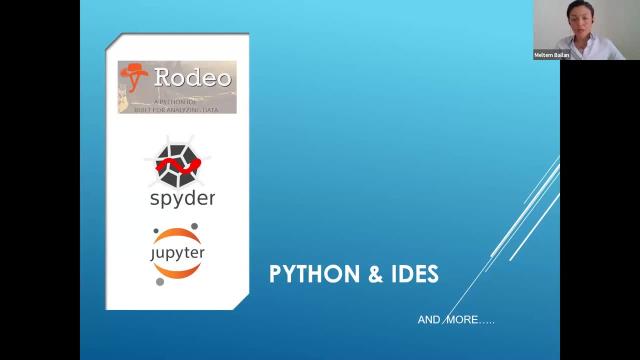 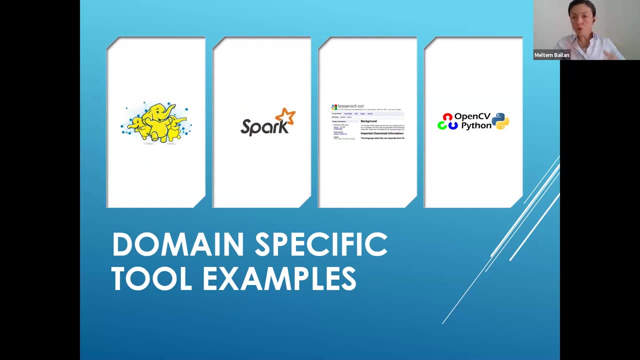 One of my favorite here is CV2.. So you can go Start your algorithms there as well. And when it comes to my projects, I leverage Tesseract for text extraction from images and OpenCV for image processing. Both are widely supported and have extensive help. 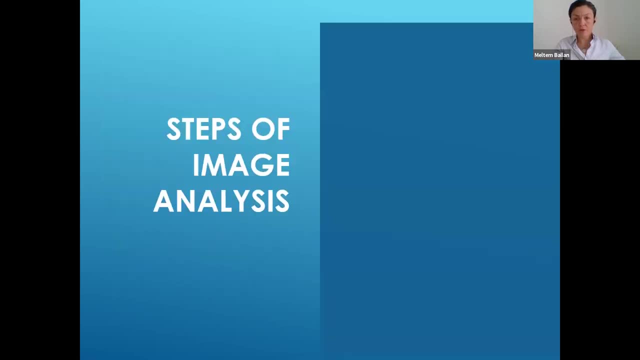 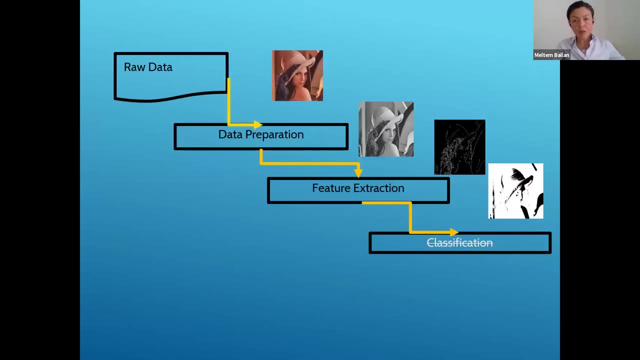 You will see some examples in the bonus material for that. As I promised, we're getting back into Lena and most used techniques in the field. There are three main steps to deal with an image. First, clean the image. then start dicing into detail that we can use in the future. 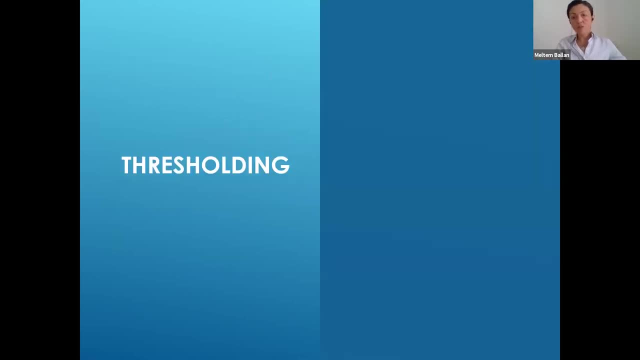 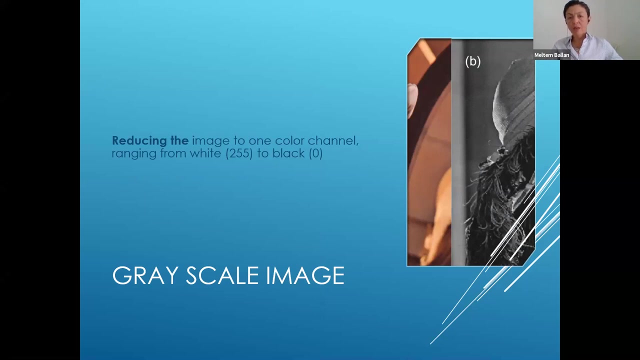 for robot vision or AI, and I will start with thresholding. It is the simplest way of separating the background from foreground. So first thing we do is to separate background from foreground And then reduce the colors. So it is called grayscaling. 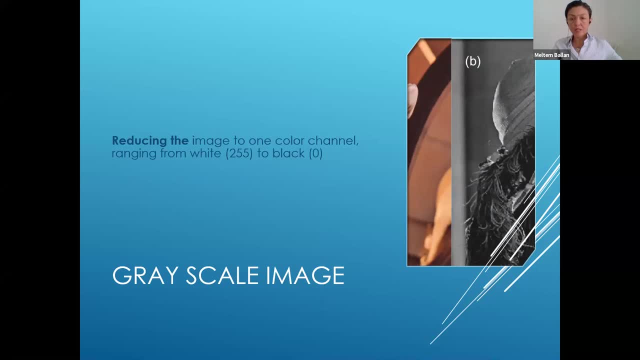 So we simply represent the image in grayscale. to begin with, This will reduce the algorithm cost And yes, even with today's technology, this is important to reduce algorithm costs. So we actually reduce the colors between black and white using a grayscaling technique. 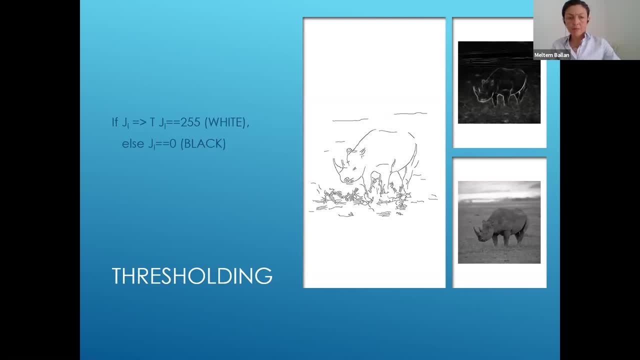 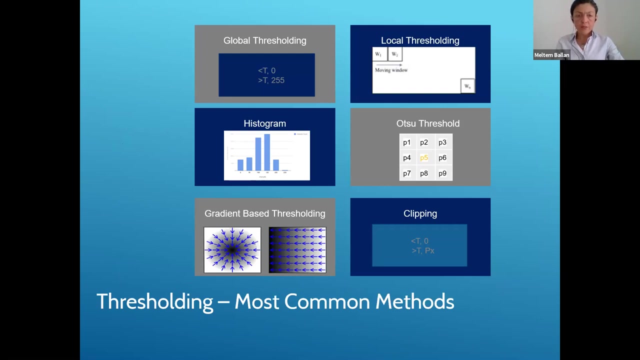 And thresholding is basically changing the color schema with a threshold value, And let me give you a couple of examples, as we have about three minutes here. The most common algorithm is global thresholding. It's the most basic implementation of that and everything else has been built like.